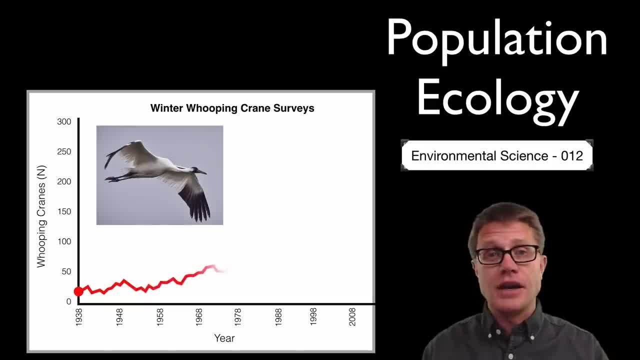 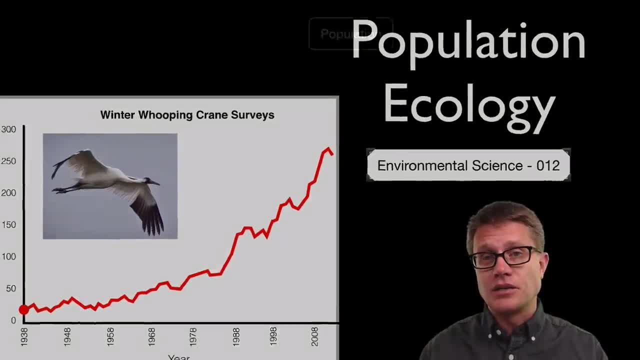 15 individuals. So scientists had to figure out: where are they, Where are they breeding? How do we protect those areas? And you can see the population is starting to rebound. But the health of the population is dependent upon the size of the population. How do we? increase the size of a population Through births and immigration, New individuals coming into the population. Likewise, how do we decrease it? Through deaths and emigration. These things contribute to what is called the intrinsic growth rate. Is it increasing or is it decreasing? 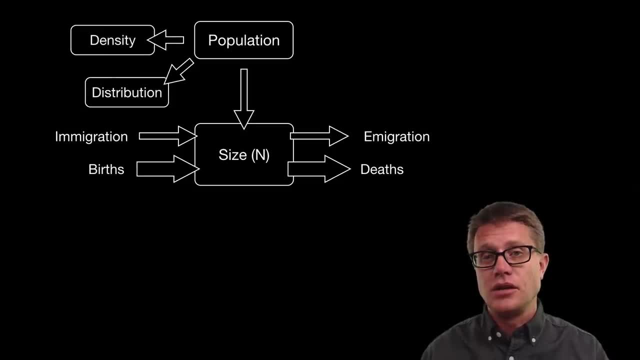 It's not the only characteristic. We also have the density and distribution. We have the sex ratio and the age structure as well. But what other factors outside of this intrinsic growth rate can affect their growth? Well, we break that into two groups: Density dependent. 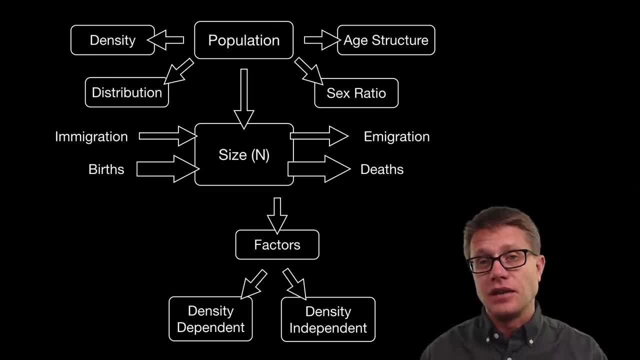 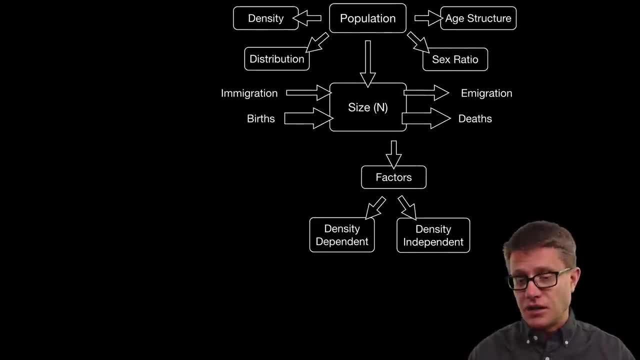 and independent Density dependent factors are factors that limit growth based on the density of the population. So, if you think about it, as the population's density increases, if there is not enough food or water or shelter, we call those limiting resources. And what? 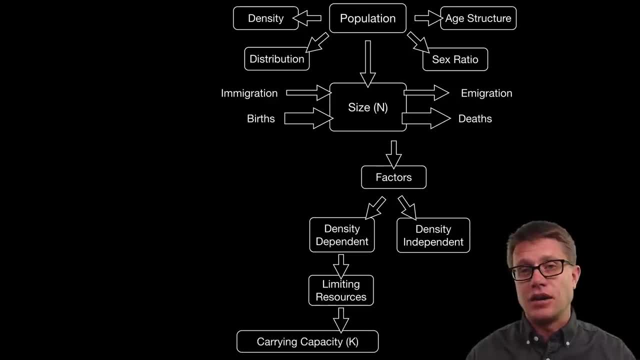 happens to the population, It will eventually level off. It hits something called a carrying capacity or K. It is the maximum number of individuals an area can support. We also have independent- And those are going to be things just related to chance- So a flood or a fire. 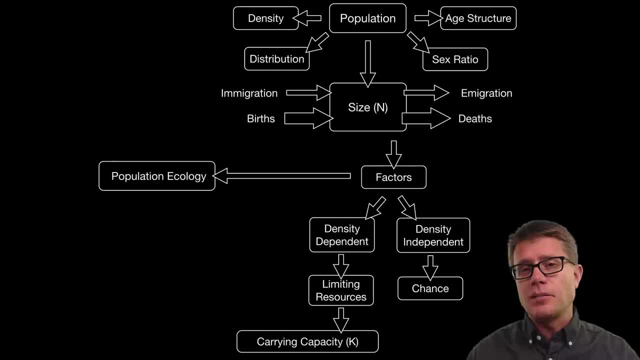 could be examples that limit the size of the population. So in population ecology we are studying these factors And scientists come up with models that help to describe what is going on in a population. So a famous model is the exponential growth model. What we are 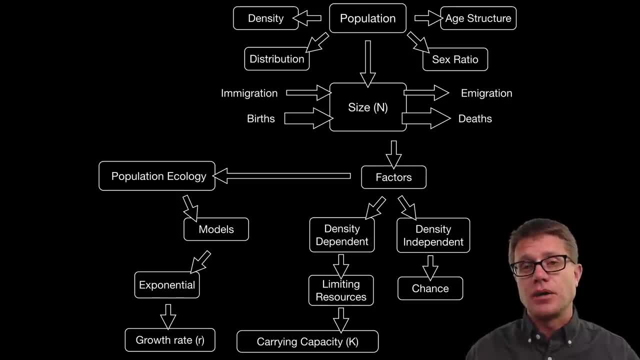 looking at is this growth rate and how it is increasing the population over time, And then we have a logistic model. It is also showing exponential growth, But eventually it is reaching what is called a density, And then we have a logistic model. It is also 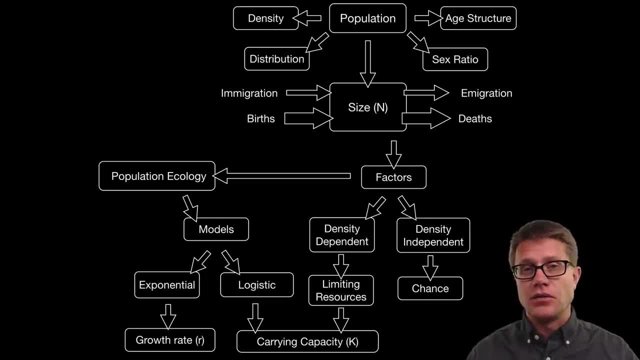 showing a carrying capacity or this limit of population growth. Scientists also study strategies that species have. Some are what are called K selected. That means their population size will increase until it gradually hits a carrying capacity And those who live more of a boom or bust cycle that are selected And we can look at how long individuals survive. 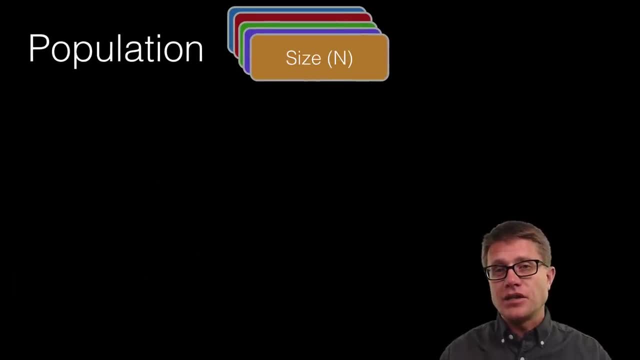 And that tells us a little bit about which strategy they are using. And so the population size is incredibly important. So if we have these rabbits, so we have 9 rabbits then if we lose 2 of them, our n value is 7.. If we gain 3 now, our n value is going to be 10.. 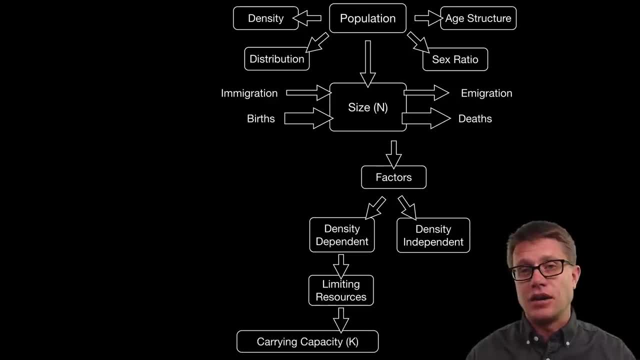 happens to the population, It will eventually level off. It hits something called a carrying capacity or K. It is the maximum number of individuals an area can support. We also have independent- And those are going to be things just related to chance- So a flood or a fire. 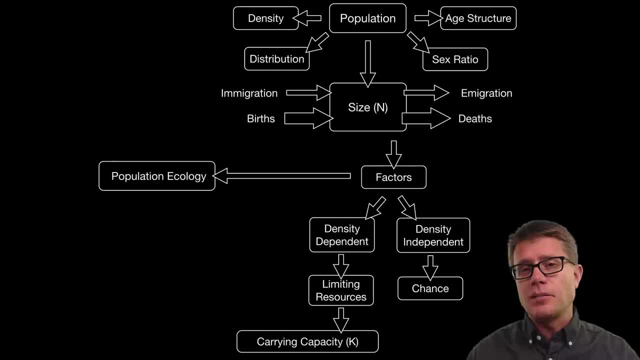 could be examples that limit the size of the population. So in population ecology we are studying these factors And scientists come up with models that help to describe what is going on in a population. So a famous model is the exponential growth model. What we are 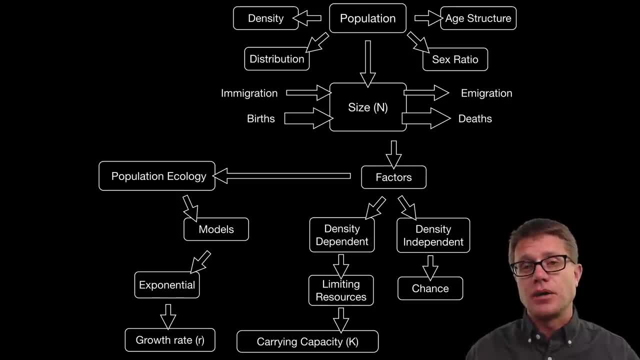 looking at is this growth rate and how it is increasing the population over time, And then we have a logistic model. It is also showing exponential growth, But eventually it is reaching what is called a density, And then we have a logistic model. It is also 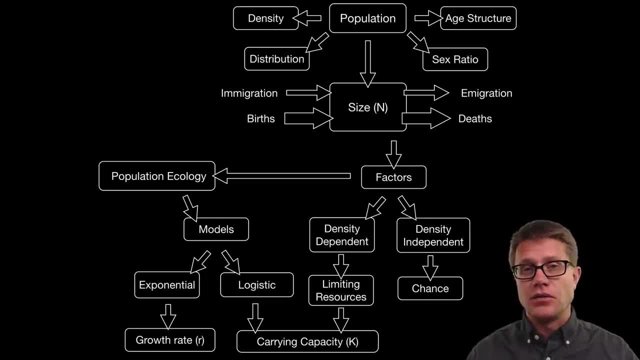 showing a carrying capacity or this limit of population growth. Scientists also study strategies that species have. Some are what are called K selected. That means their population size will increase until it gradually hits a carrying capacity And those who live more of a boom or bust cycle that are selected And we can look at how long individuals survive. 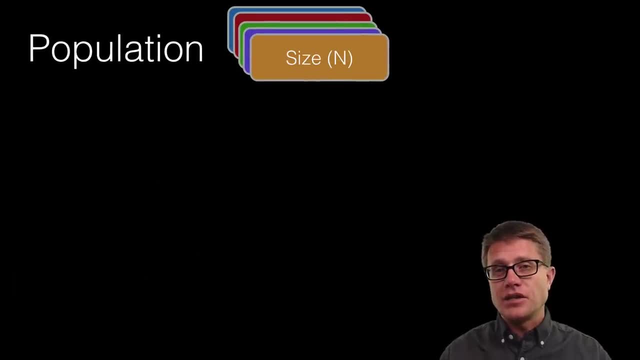 And that tells us a little bit about which strategy they are using. And so the population size is incredibly important. So if we have these rabbits, so we have 9 rabbits then if we lose two of them, our n value is 7.. If we gain 3 now, our n value is going to be 10.. 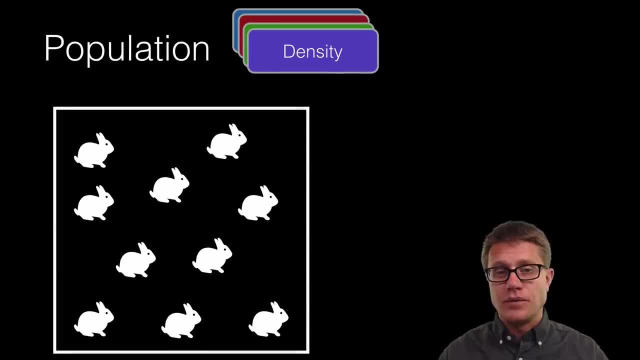 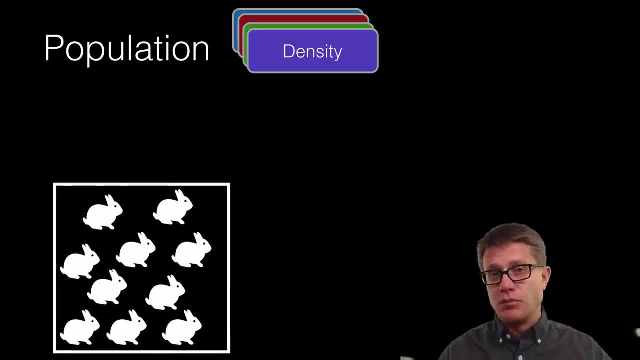 It is the set number we have, But also density is important. That is, the number of individuals we have in a given area, And so we could call this one density, But we would call this greater density. We could also look at their distribution. I would say that these rabbits are now randomly. 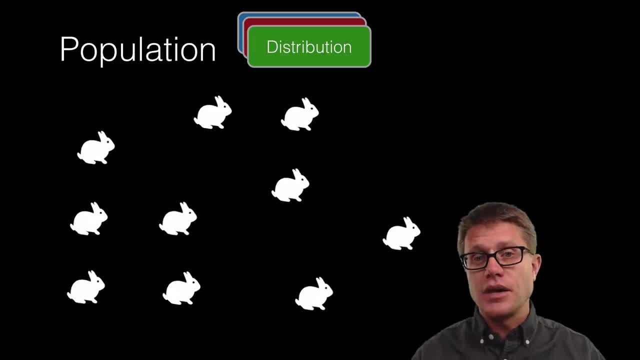 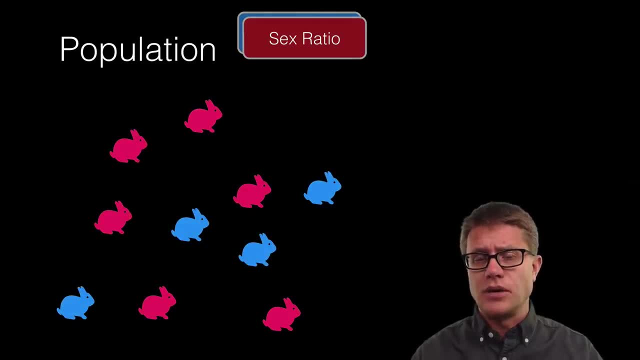 distributed, But they could be distributed uniformly Or they could just be clumped in their distribution And we could also look at their sex ratio, So how many of our males, how many of them are going to be females. And we could expand that to look at what is. 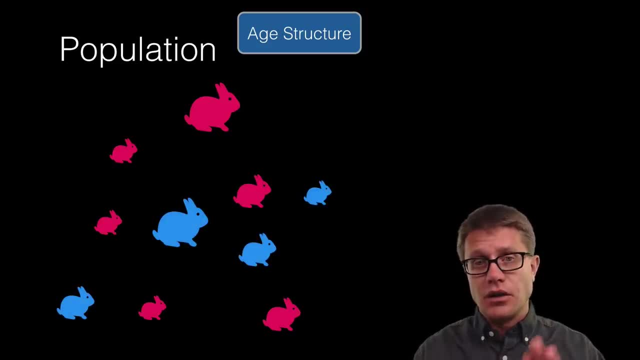 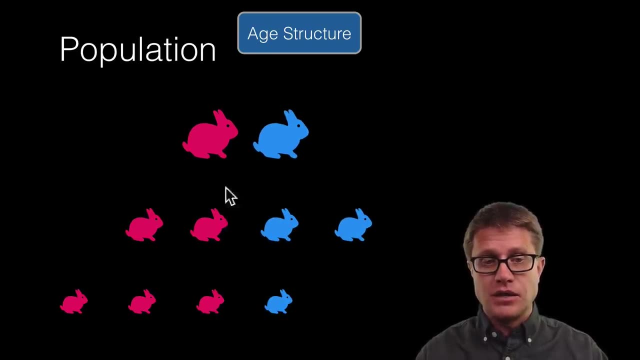 called their age structure: Not only what is their gender, but also how old are they. So we could organize them like this: where this is going to be our first year, female rabbit, second year and third year, And we can do the same thing with males, But when. 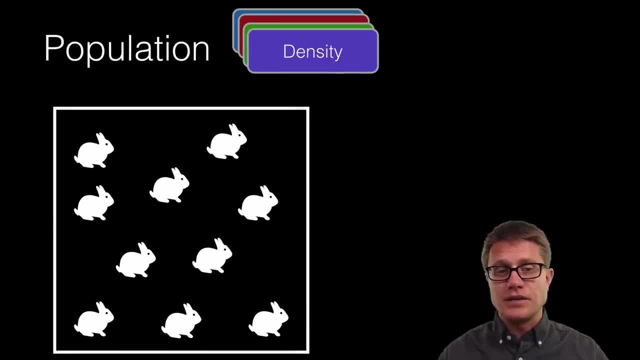 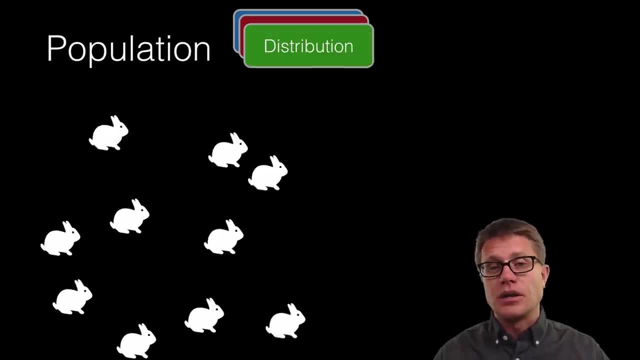 It is the set number we have, But also density is important. That is, the number of individuals we have in a given area, And so we could call this one density, but we would call this greater density. We could also look at their distribution. I would say that these rabbits are now randomly. 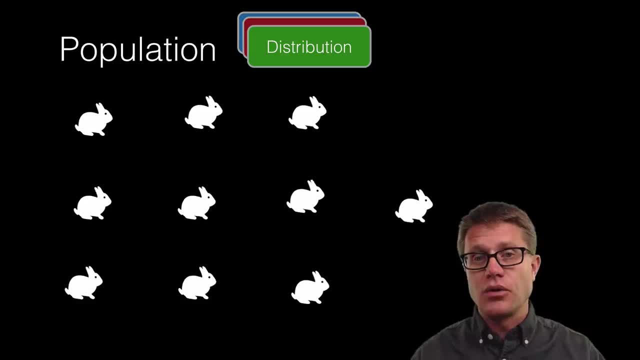 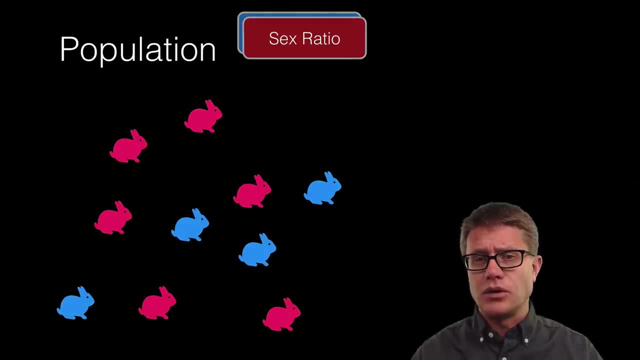 distributed, but they could be distributed uniformly Or they could just be clumped in their distribution And we could also look at their sex ratio, So how many of our males, how many of them are going to be females. And we could expand that to look at what is. 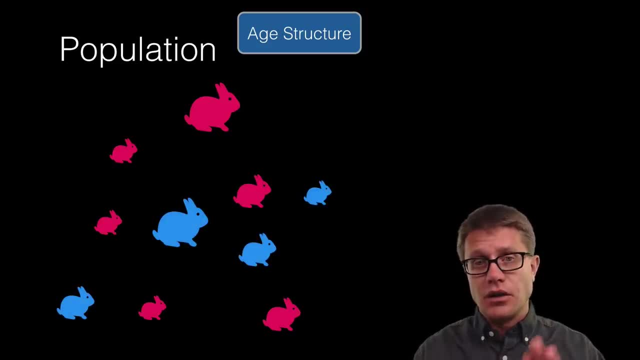 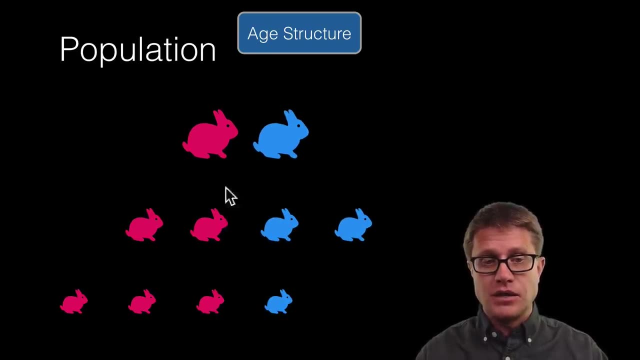 called their age structure: Not only what is their gender, but also how old are they. So we could organize them like this: where this is going to be our first year, female rabbit, second year and third year, And we can do the same thing with males, But when. 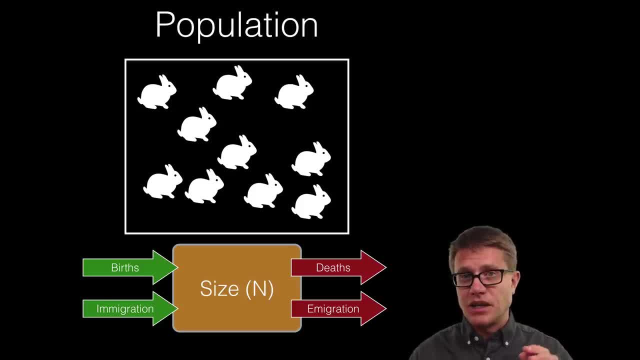 it comes to the health. the population size is incredibly important. It is dictated by births, deaths, immigration and emigration, And so we have a formula that allows us to look at that, And the calculations are very simple. You can do them just in your head. 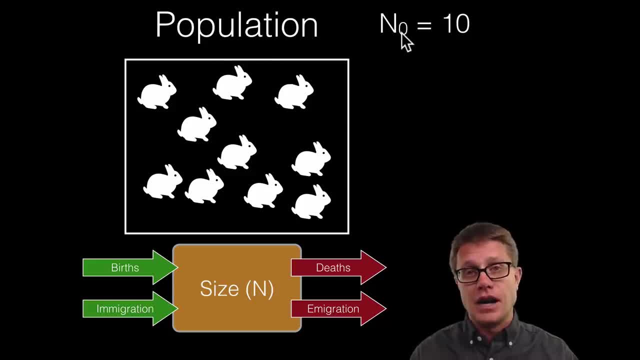 And so let's say we have a population of 10.. So our n naught is going to be 10.. That is our initial population. Here is our equation. So it is really simple. The change in n is going to be the births minus the deaths, plus the immigration, minus the emigration. So let's 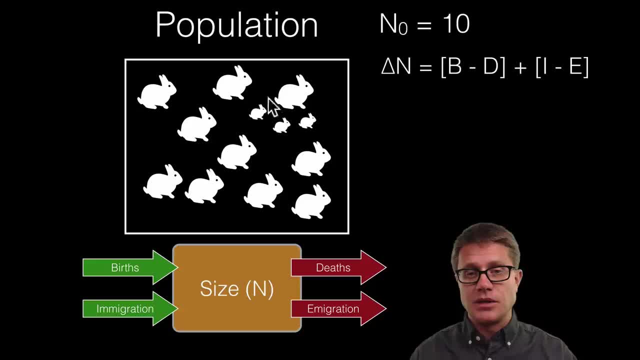 look at this population over here and see what happens. So this rabbit gave birth to three other rabbits, And so, if we write this out, what is our births going to be? It is going to be 10.. So we have the population of 10.. So what we are going to do is we are 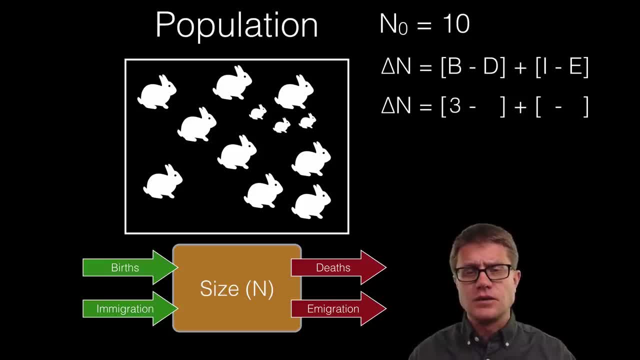 going to put a 1 here in the deaths. We could look at immigration: How many come in? Looks like just one, So we would put a 1 right here. And then how many emigrate? It looks like two left, And so we would put a 2 right here, And so the delta n, or the change in n, is simply 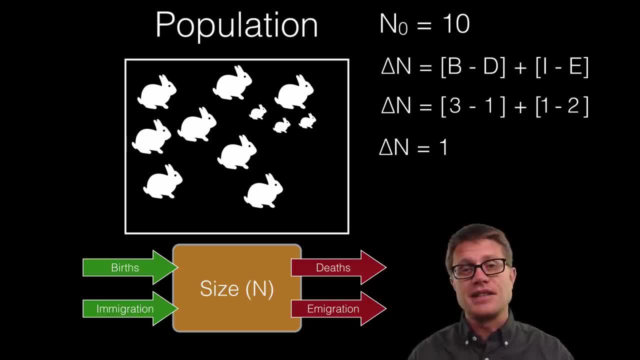 going to be 3 minus 1, plus 1 minus 2 or 1.. That is the change, Or we have seen an increase in 1.. Now what is the growth rate? The growth rate is going to be the change divided by the initial population. So 1 divided by 10 gives 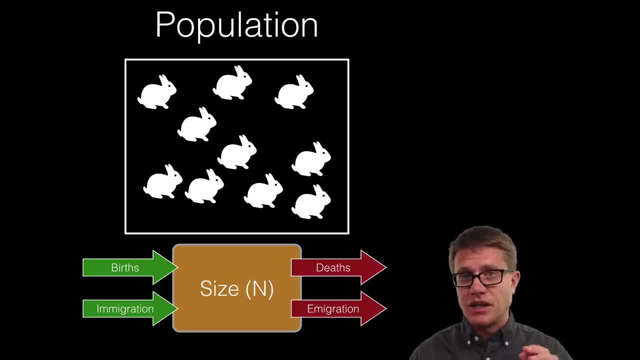 it comes to the health. the population size is incredibly important. It is dictated by births, deaths, immigration and emigration, And so we have a formula that allows us to look at that, And the calculations are very simple. You can do them just in your head. 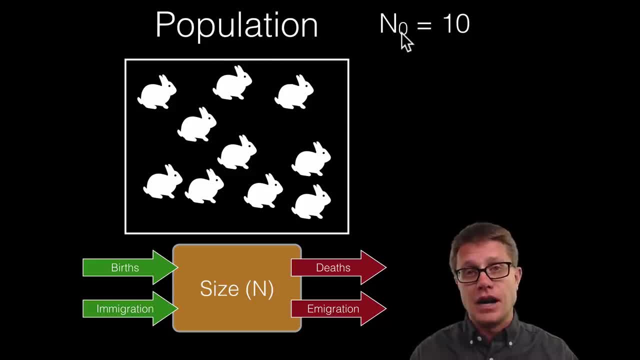 And so let's say we have a population of 10.. So our n0 is going to be 10.. That is our initial population. Here is our equation. So it is really simple. The change in n is going to be the births minus the deaths, plus the immigration, minus the emigration. So let's look at this. 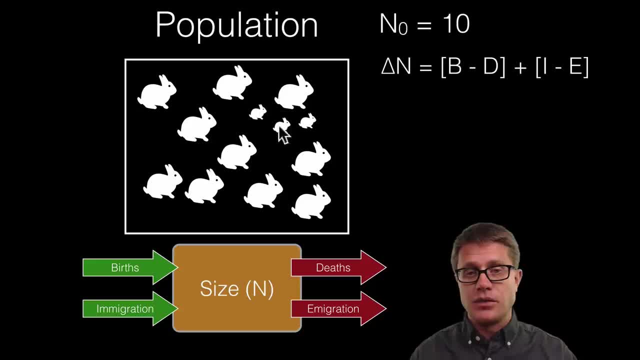 population over here and see what happens. So this rabbit gave birth to three other rabbits, And so if we write this out, what is our births going to be? It is going to be three other rabbits. Now let's watch the population again So you can see: one of the rabbits died And 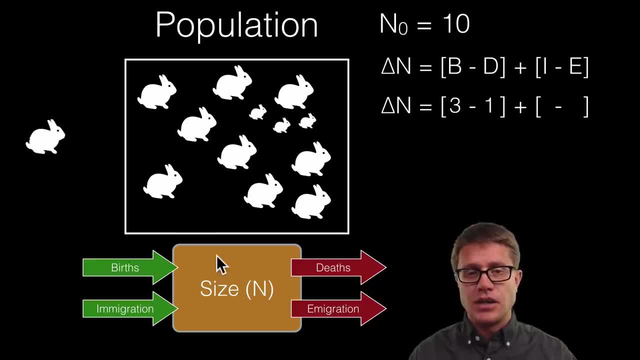 so we are going to put a 1 here in the deaths. We could look at immigration. How many come in? It looks like just one, So we would put a 1 right here. And then how many emigrate? It looks like two left, And so we would put a 2 right here. And so the delta n or the 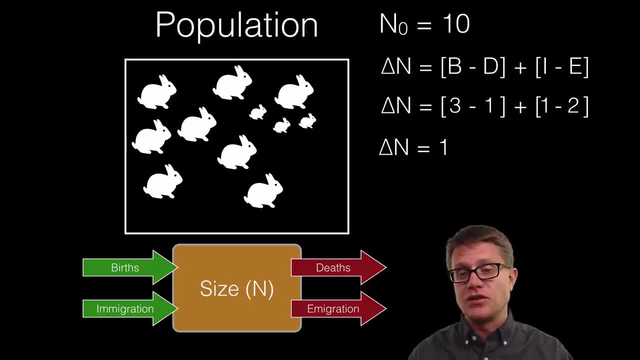 change in n is simply going to be 3 minus 1 plus 1 minus 2 or 1.. That is the change, Or we have seen an increase in 1.. Now what is the growth rate? The growth rate is going to be the change divided by the initial population. So 1 divided by 10 gives us a 10% growth rate. 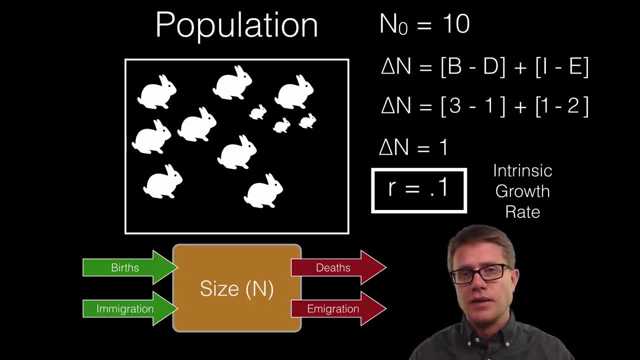 Or 0.1 is our growth rate. We call that the intrinsic growth rate And as long as we have no other factors outside that population, that will remain constant over time. And you could solve a really hard problem. If we have a million people in an area, 100,000 are born. 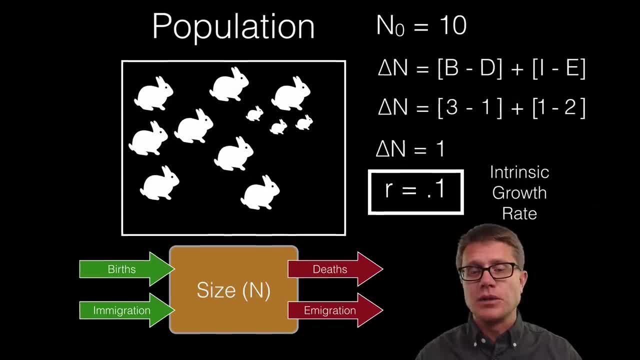 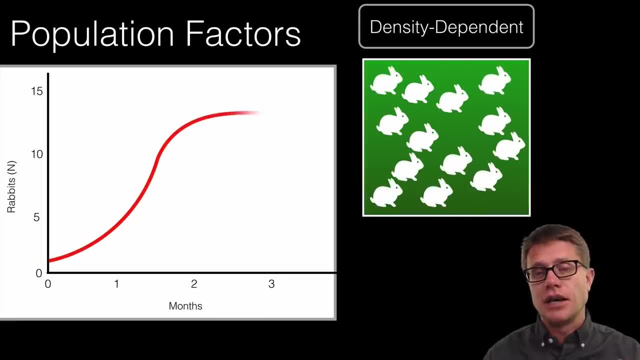 10,000 die. If you are given the immigration and emigration, you should be able to calculate r for that population. So if we study a group of rabbits, over time their population will increase, But it will eventually level out at some point. Now that leveling out point. 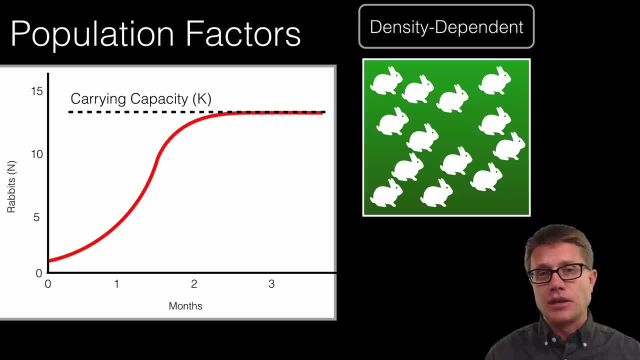 is called the carrying capacity or the k. Now why is a population going to level out? It is because they are running out of something. They are running out of food or water or shelter, And so we call all of those things limiting resources. Disease could be another limiting 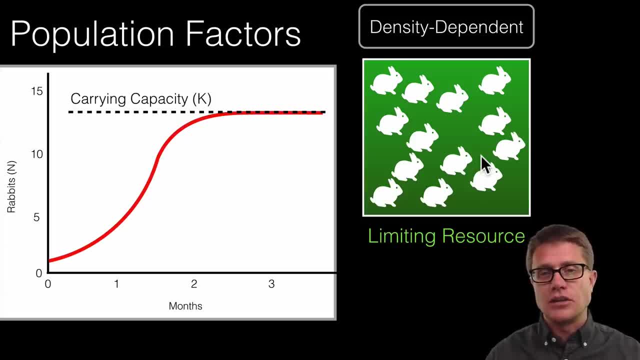 resource. The more rabbits we have, the more disease, And so it is eventually going to level it off. Now it will not look perfect like that In a normal population. it is going to have overshoots And it is going to have a lot of die off, But we are going to have 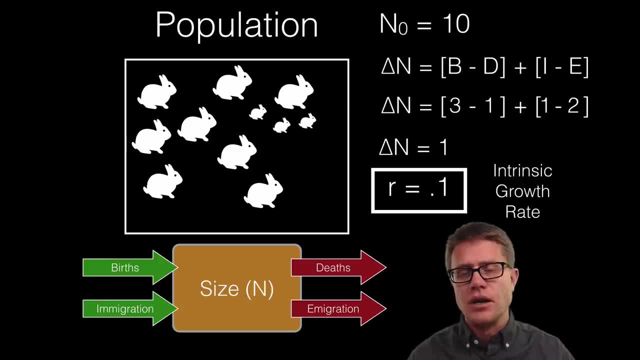 us a 10 percent growth rate, Or .1 is our growth rate. We call that the intrinsic growth rate And as long as we have no other factors outside that population, that will remain constant over time And you could solve a really hard problem If we have a million people in an 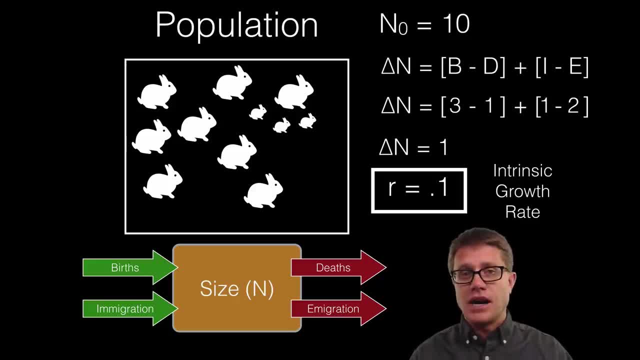 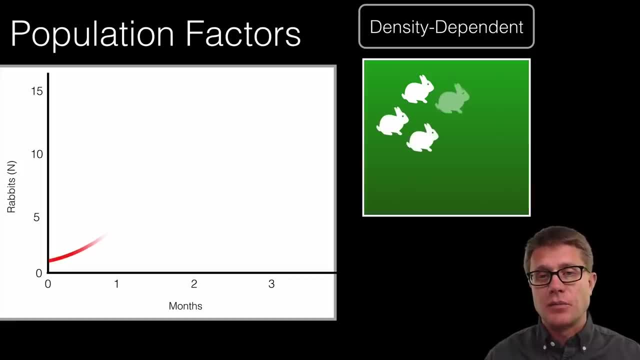 area, 100,000 are born, 10,000 die. if you are given the immigration and emigration, you should be able to calculate r for that population. So if we study a group of rabbits, over time population will increase but it will eventually level out at some point. Now that leveling 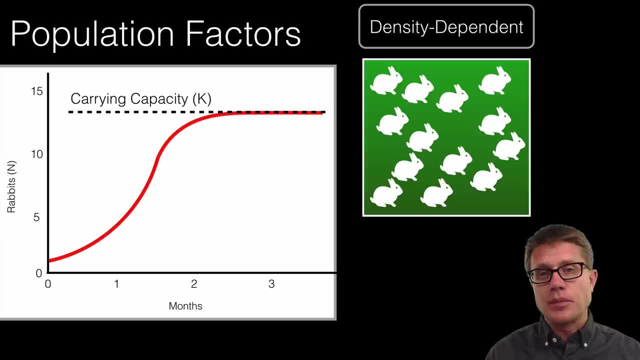 out point is called the carrying capacity or the K. Now why is the population going to level out? It is because they are running out of something. They are running out of food or water or shelter, And so we call all of those things limiting resources Disease. 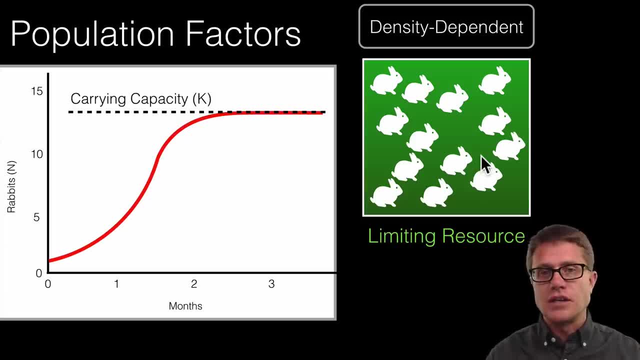 could be another limiting resource. The more rabbits we have, the more disease, and so it is eventually going to level it off. Now it will not look perfect like that In a normal population. it is going to have overshoots and it is going to have a lot of die off. 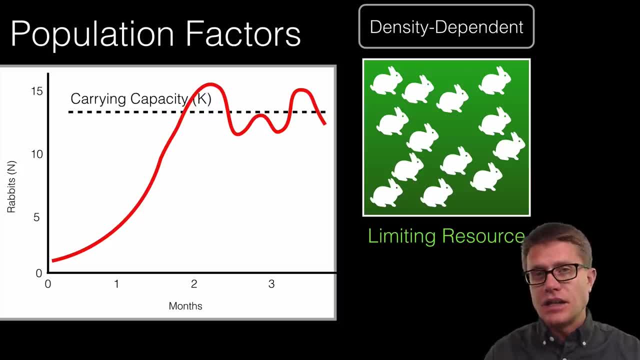 But we are going to have that average that we eventually hit. These are density dependent factors because they are based on the density of the population. We can also have density independent. So imagine that these rabbits over on this side are killed in a forest fire. 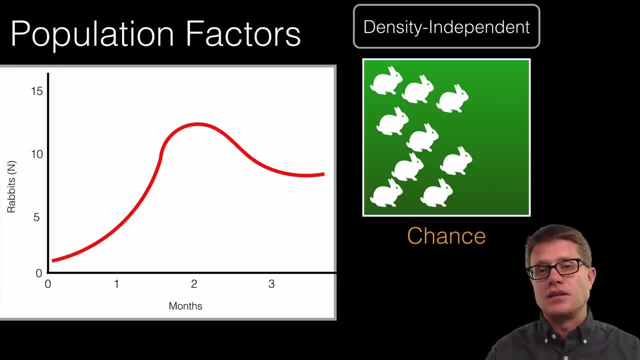 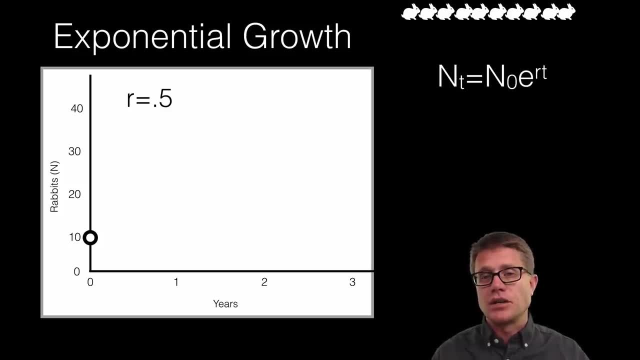 That is just chance. It is just chance taking over, And so it is not based on the density of rabbits that we had. So if we start to use models to explain how this works, a really important model is the exponential growth model, And so the equation looks like this. It is a little scary, but it is really not that bad. 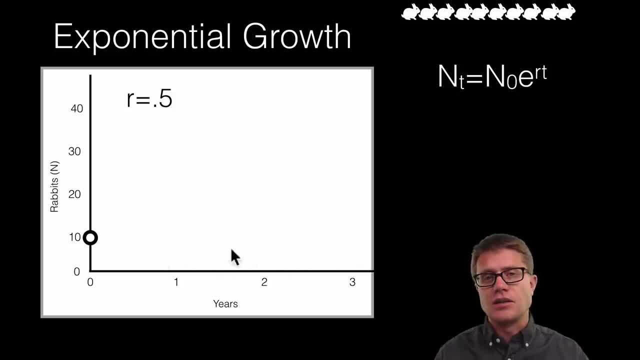 N sub T is going to be the population at any time into the future. N sub O is going to be the initial population. So let's say we start with a population of 10.. R is going to be the growth rate, That is that intrinsic growth rate, And T is going to be time. So 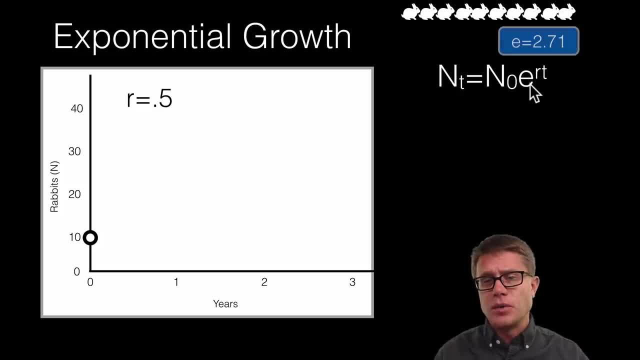 the only thing that you really do not know in this equation is E. E is going to be E, the mathematical constant. So it is a number. It is just like pi: It is going to be 2.718.. It just keeps going like that. 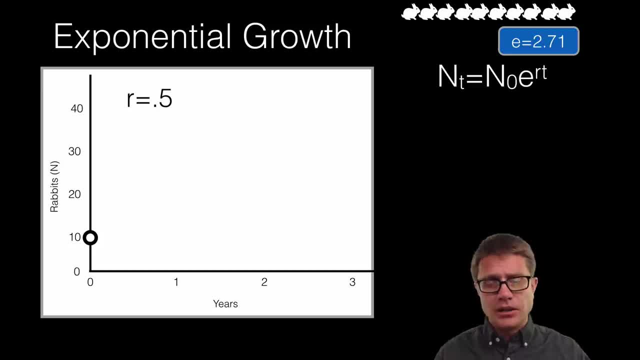 So for our purposes we just think of it as 2.71.. And so let's say we want to figure out what is going to happen to the population in year 1.. So if we want to figure out- we started at 10,- what is going to be the population Probably at year 1.. We just use this equation. 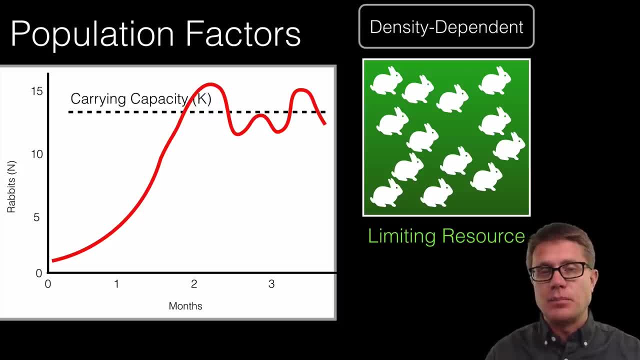 that average that we eventually hit. These are density dependent factors because they are based on the density of the population. We can also have density independent, So imagine that these rabbits over on this side are killed in a forest fire. That is just chance It. 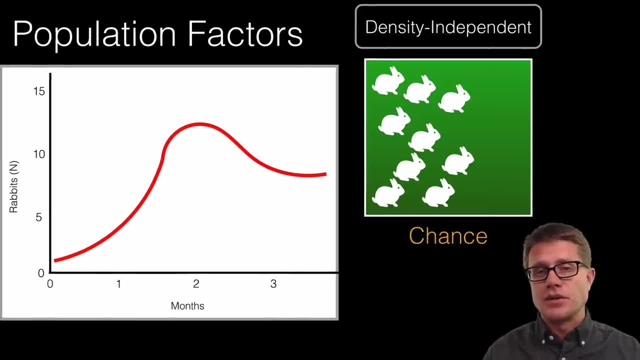 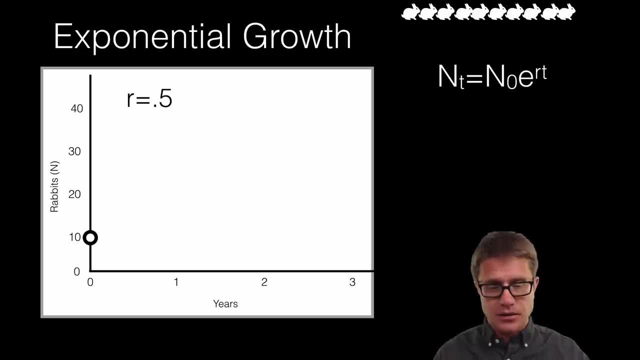 is just chance taking over, And so it is not based on the density of rabbits that we had. So if we start to use models to explain how this works, a really important model is the exponential growth model, And so the equation looks like this. It is a little scary, but 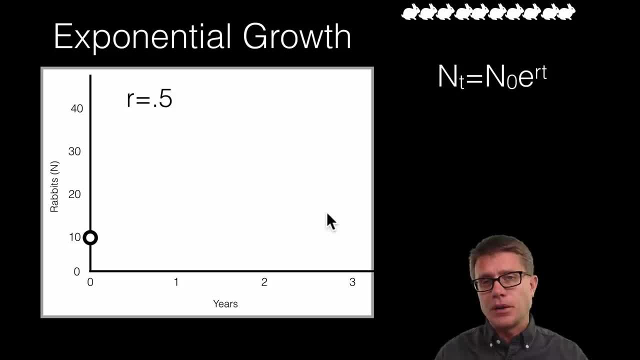 it is really not that bad. N sub t is going to be the population at any time into the future. N sub o is going to be the initial population. So let's say we start with a population of 10.. R is going to be the growth rate, That is that intrinsic growth rate, And t is going to be time. So 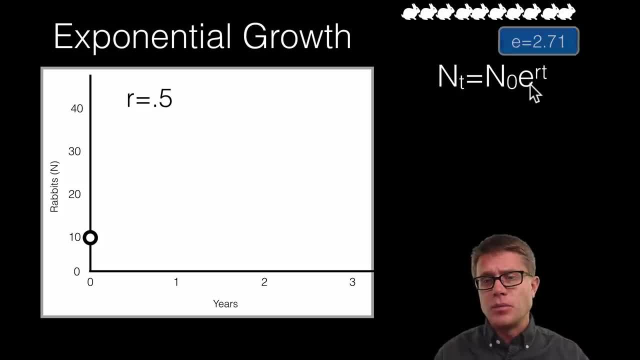 the only thing that you really do not know in this equation is e. e is going to be e, the mathematical constant. So it is a number. It is just like pi. It is going to be 2.718.. It just keeps going like that. So for our purposes, we just think of it as 2.71.. And 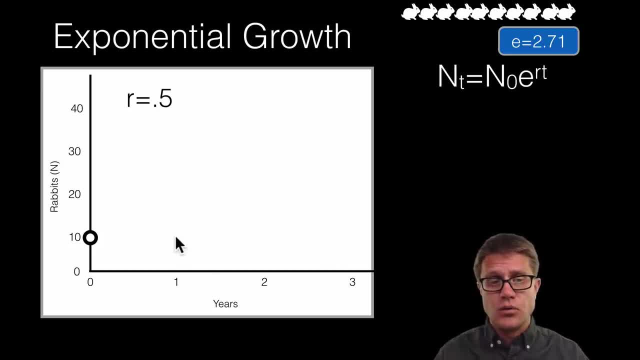 so let's say we want to figure out what is going to be the population at any time into the future. What is going to happen to the population in year 1? So if we want to figure out- we started at 10, what is going to be the population probably at year 1? We just 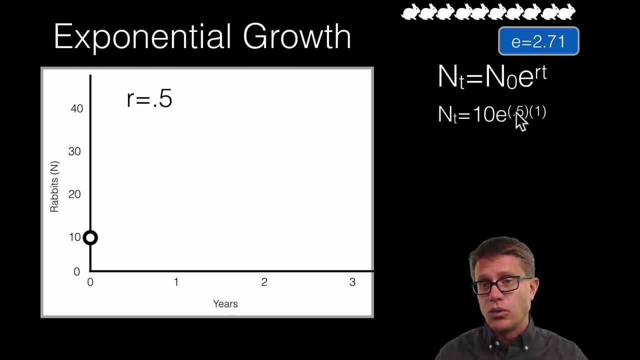 use this equation. So e is going to be the same. So what is going to be our r value? Our r value will always be 0.5.. That is that intrinsic growth rate. What is our t value? Our t value is going to be time. What is our initial population? It is going to be 10.. 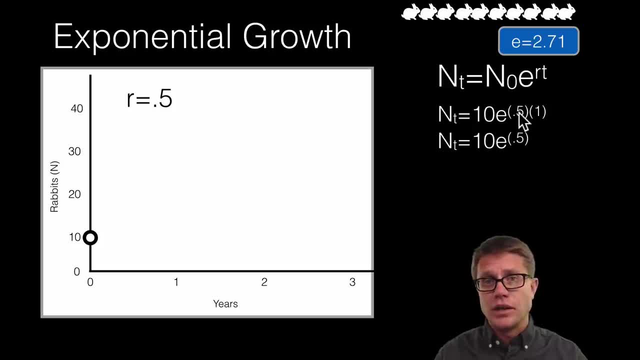 So if I expand that a little bit, we are simply multiplying 1 times 0.5, one year times that growth rate, And so that is going to be 10 times 2.71.. Again, that is e raised to the 0.5 power. 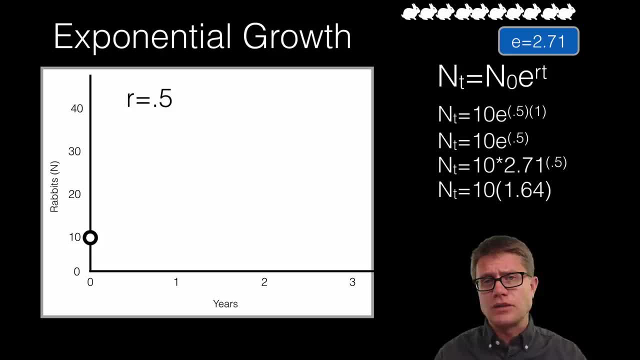 So that is really like taking the square root of 2.71.. And so that is 1.64.. So if we work that out, that is going to be around 16 rabbits after one year. So let me graph that and let's. 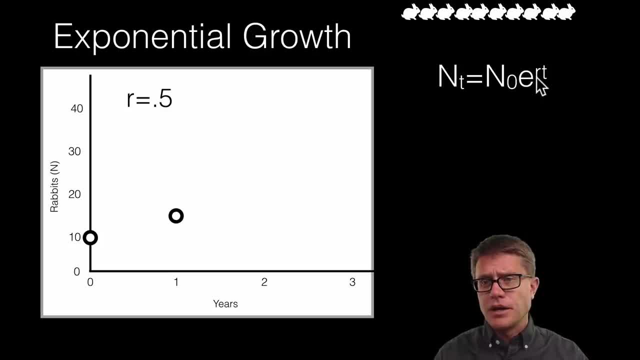 go to year 2.. So same thing: We are going to plug in our value of 0.5, but now our t value is going to be 2.. We still have that same initial population. And so now we are going to have the same initial population. We are going to have the same initial population. 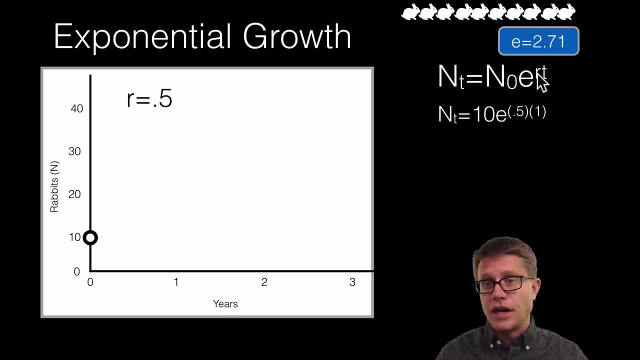 So E is going to be the same. So what is going to be our R value? Our R value will always be 0.5. That is that intrinsic growth rate. What is our T value? Our T value is going to be time. What is our initial population? It is going to be 10.. So if I expand that a 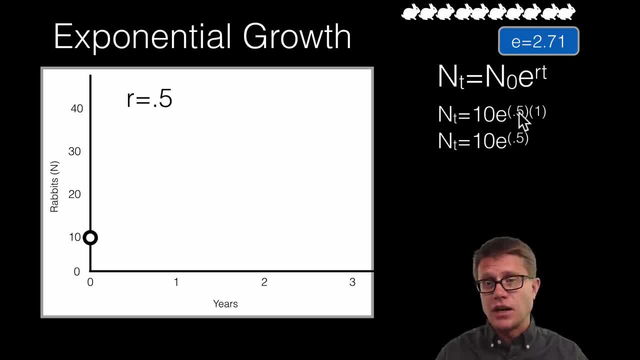 little bit. we are simply multiplying 1 times 0.5, 1 year times that growth rate, And so that is going to be 10 times 2.71.. Again, that is E raised to the 0.5 power. So that is really. 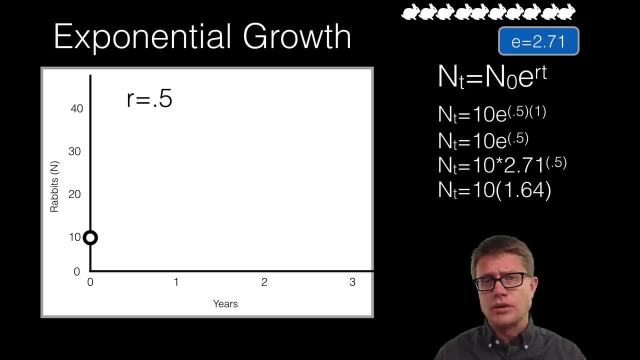 like taking the square root of 2.71.. And so that is 1.64.. So if we work that out, that is going to be around 16 rabbits after 1 year. So let me graph that And let's go to year. 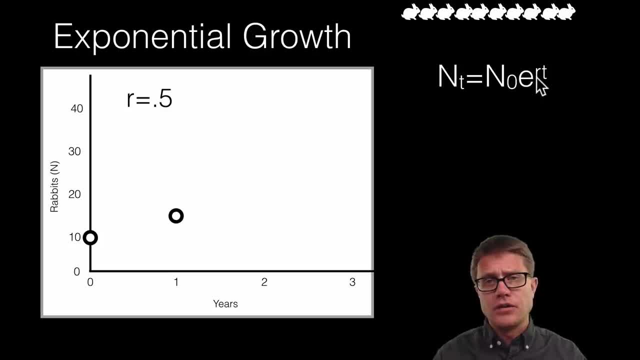 2.. So same thing. We are going to plug in our value of 0.5. But now our T value is going to be 2.. Still have that same initial population, And so now it is going to be 2.71 raised to. 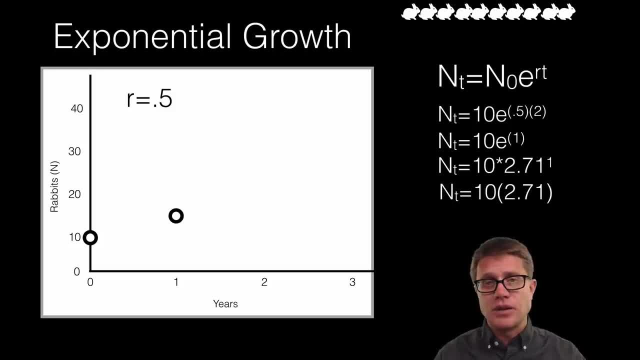 the 1 power. So what is that? That is simply 2.71.. So if we work this out now, we are going to have 27 rabbits in that next year. You can see the population is increasing. We are starting to see that exponential growth. Let's go for year 3.. So if we figure out year 3 again, 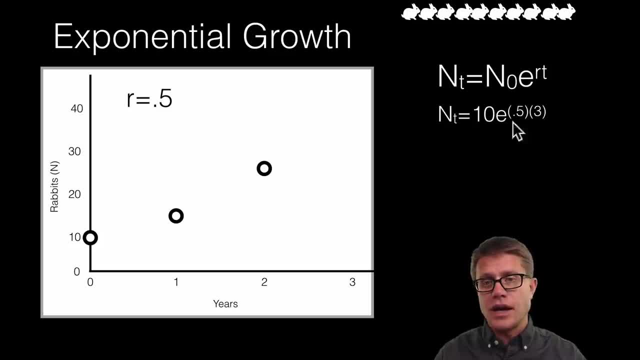 Our intrinsic growth rate is still 0.5.. 3 is going to be the year we are at, Still have that same initial, And so this is going to be 2.71 raised to the 1.5 power. You probably need a calculator. 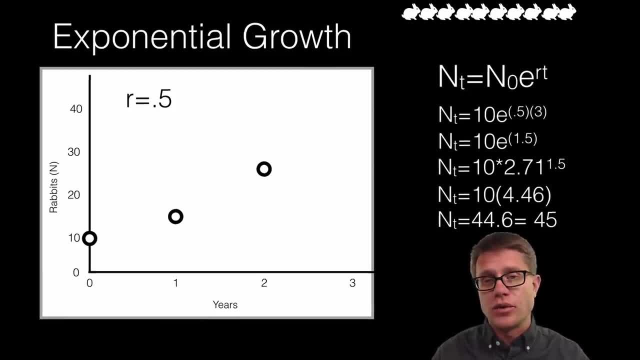 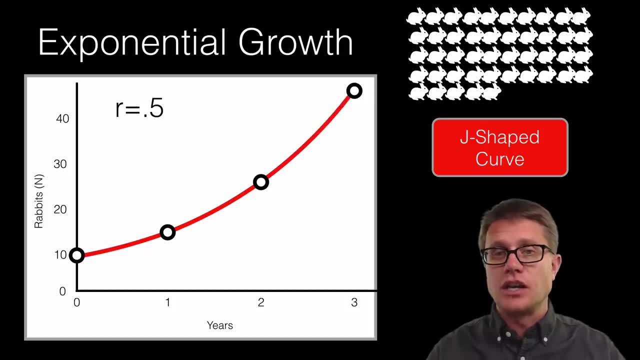 to do this, We now get 44.6, or let's say 45 rabbits. So if we graph it, you can see that the population is increasing. like that, We have what is called a J shaped curve And it is going to increase rapidly over time. We are going to the whole world would be. 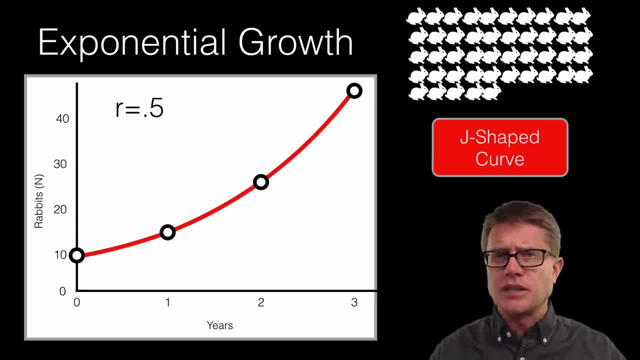 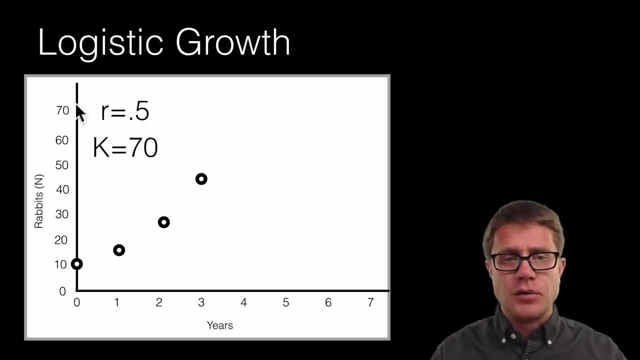 filled with rabbits if we keep following this model And so we know that is not what occurs, And so not only intrinsic growth rate is important, but K, that carrying capacity. So if you are given a problem like this, could you graph what is going to happen over time If K is? 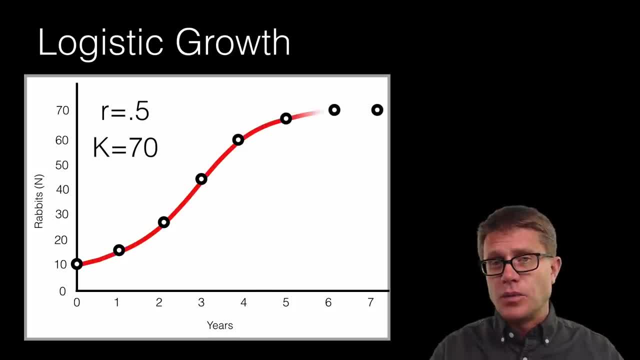 70,. well, you are going to get something that looks like this: It is going to be J for a while, but it is eventually going to curve off and we are going to have an S shaped curve. This is a logistic growth model. There is also a mathematical model. we will not work. 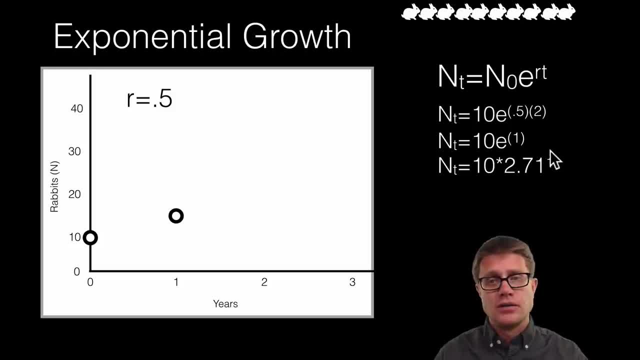 So now it is going to be 2.71 raised to the 1 power. So what is that? That is simply 2.71.. So if we work this out now, we are going to have 27 rabbits in that next year. You. 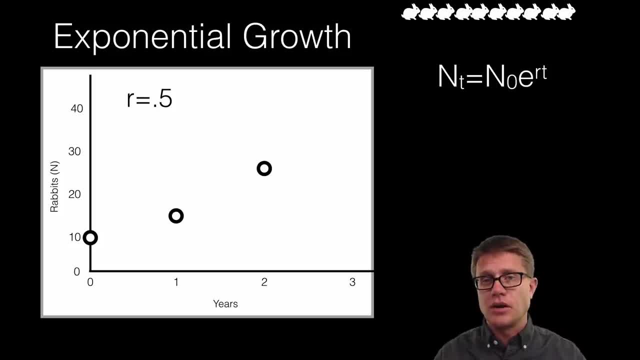 can see, the population is increasing. We are starting to see that exponential growth. Let's go for year 3.. So if we figure out year 3 again, our intrinsic growth rate is still 0.5.. Three is going to be the year we are at. We still have that same initial And so 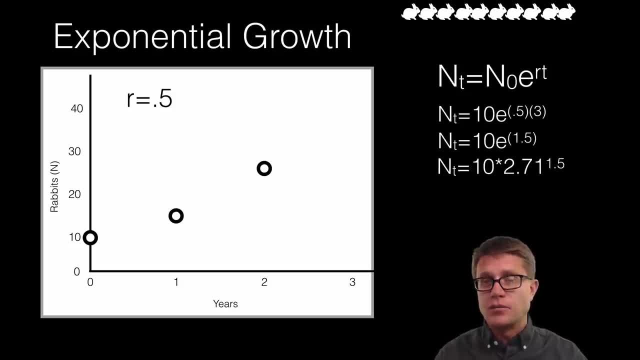 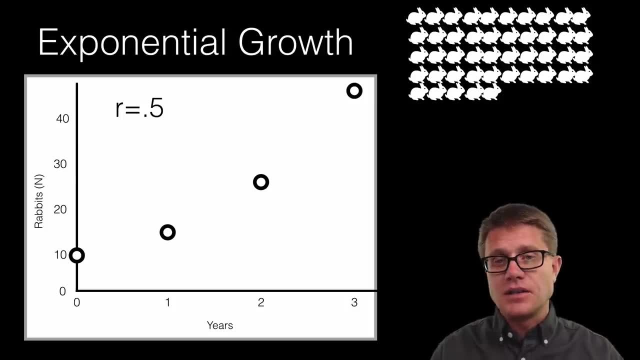 this is going to be 2.71 raised to the 1.5 power. You would probably need a calculator to do this. We now get 44.6, or let's say 45 rabbits. So if we graph it, you can see that. 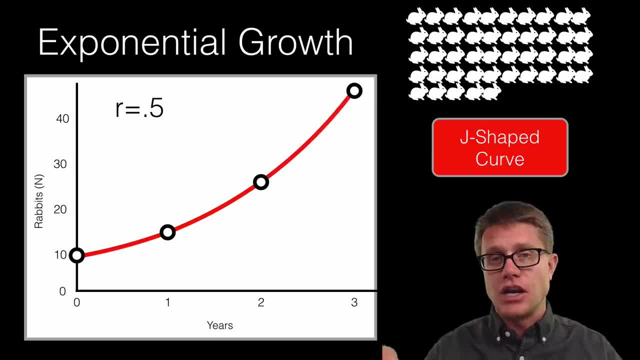 the population is increasing like that. We have what is called a J shaped curve, And it is going to increase rapidly over time We are going to the whole world would be filled with rabbits if we keep following this model, And so we know that is not what occurs. 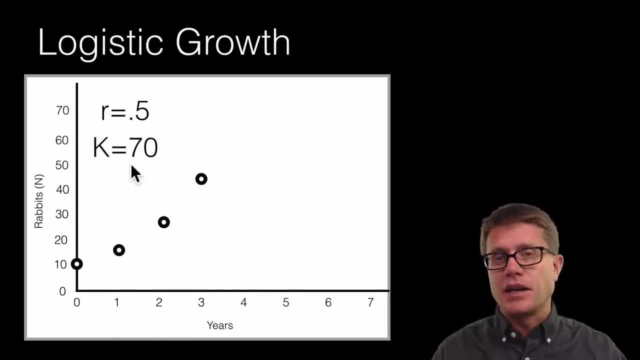 And so not only intrinsic growth rate is important, but k, that carrying capacity. So if you are given a problem like this, could you graph what is going to happen over time if, for example, if k is 70, well, you are going to get something that looks like this: It is. 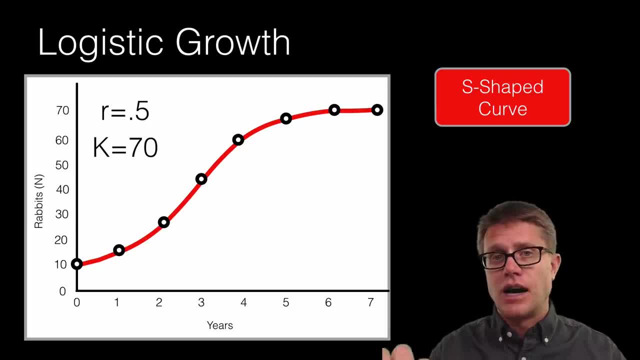 going to be J for a while, but it is eventually going to curve off and we are going to have an S shaped curve. This is a logistic growth model. There is also a mathematical model we will not work through. I will put a link to another video where I do that down below. 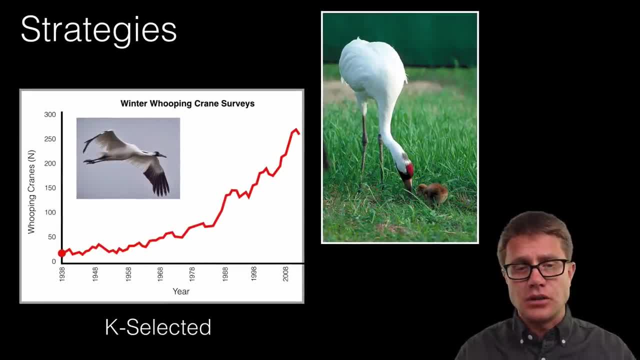 And so scientists, now that they have models, they can start to apply that to nature. So what we have found is that species kind of fall into one of two camps. We have what are called k selected species. Those are going to be species that their population is going. 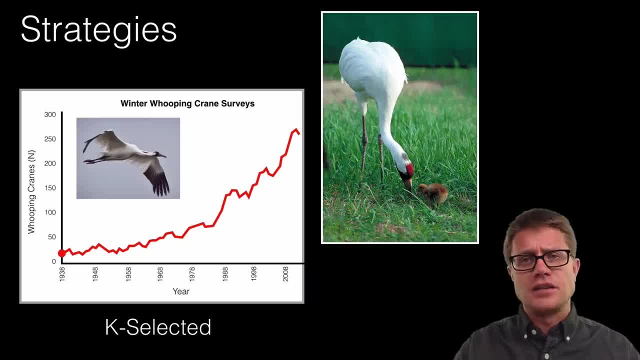 to increase and then it will eventually hit a carrying capacity and it stays there. What are some characteristics of species like that? They are going to give a lot of parental care to their offspring. They are just going to have a few offspring, And so the whooping. 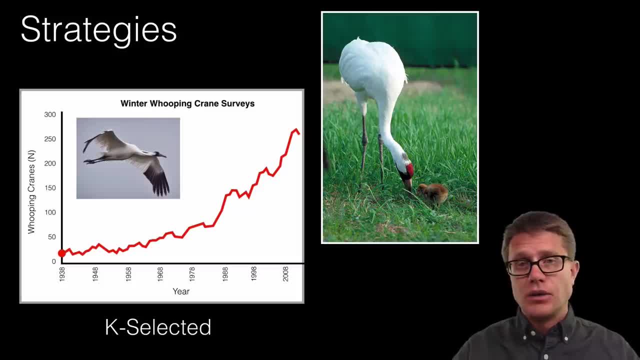 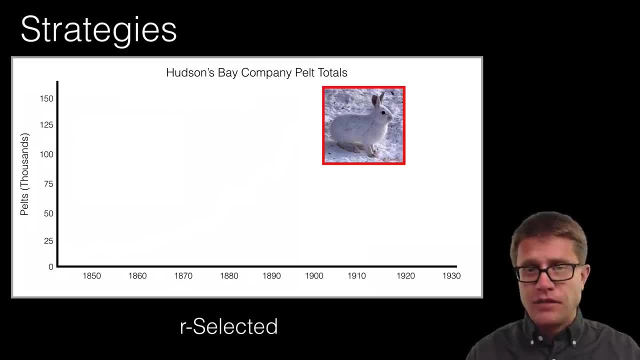 crane would be an example of that. Humans are an example of that. We do not just go up and down in our population. R selected are going to do that. So an arctic hare is an example of that. A famous study was looking at the pelts that were collected by the Hudson. 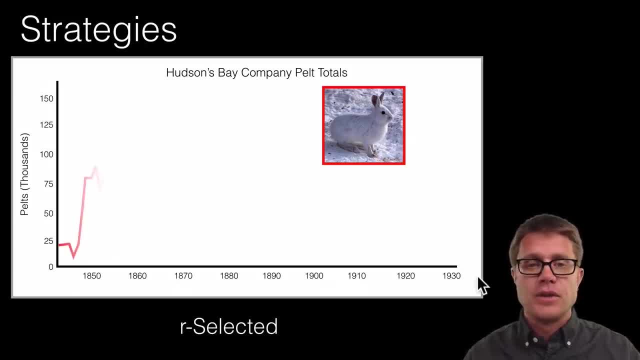 Bay Company And they found from 1850 to 1930 that the population of arctic hare just went up and down and up and down. And so hares are going to be groups of individuals that have lots of offspring. They do not get tons of parental care And 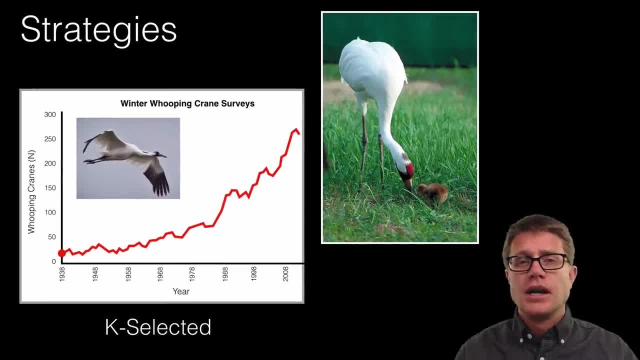 through. I will put a link to another video where I do that down below. And so scientists, now that they have models, they can start to apply these models. And so scientists, now that they have models, they can start to apply these models. And so scientists, now that they have models, they can start to apply. 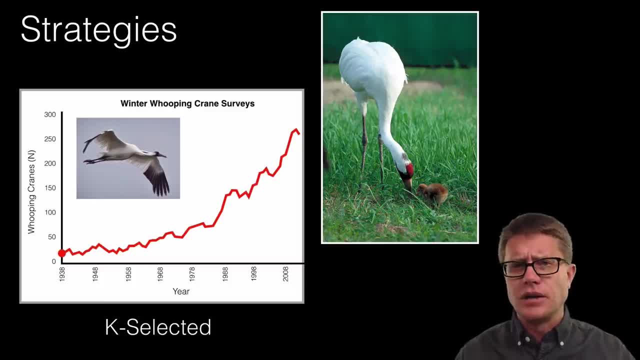 that to nature. So what we found is that species kind of fall into one of two camps. We have what are called K selected species. Those are going to be species that their population increases and then it will eventually hit a carrying capacity and it stays there. What? 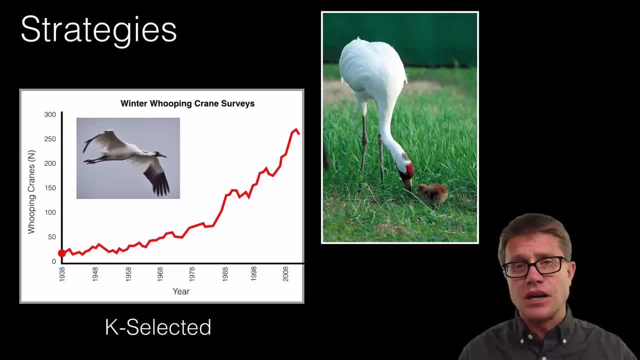 are some characteristics of species like that. They are going to give a lot of parental care to their offspring. They are just going to have a few offspring, And so the whooping crane would be an example of that. Humans are an example of that. We do not just go. 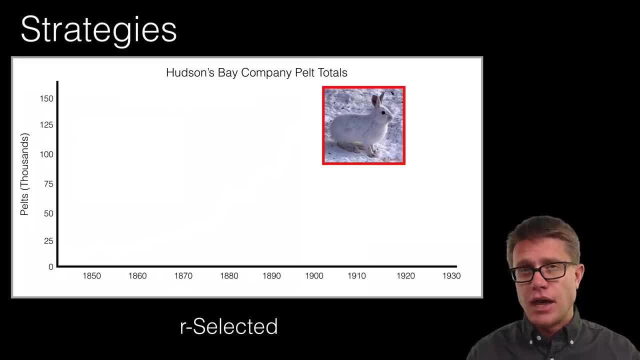 up and down in our population, R selected are going to do that. So an Arctic hare is an example of that. A famous study was looking at the pelts that were collected by the Hudson Bay Company And they found from 1850 to 1930 that the population of Arctic 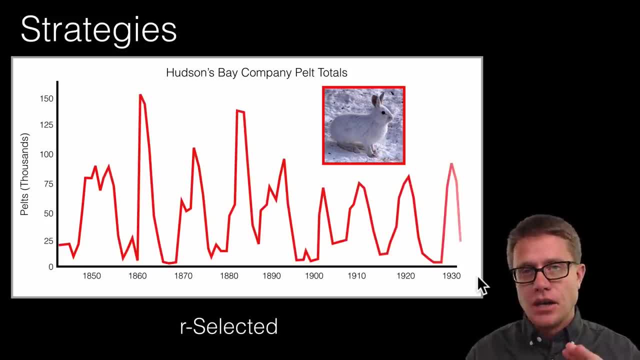 hares just went up and down and up and down, And so hares are going to be groups of individuals that have lots of offspring, They do not get tons of parental care And their population is going to increase, and then it will crash. So we have this boom and bust cycle. Now what? 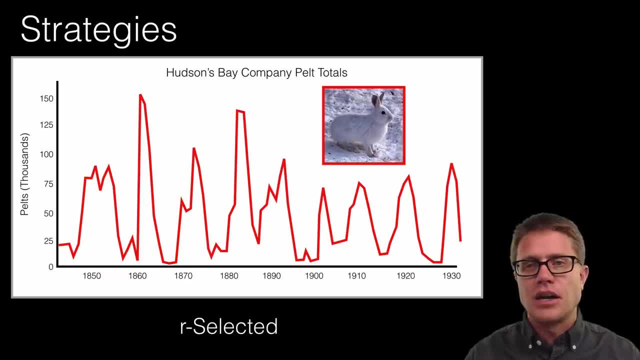 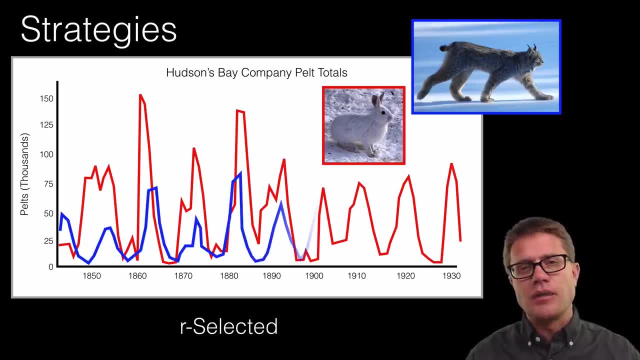 is interesting is that there is another species, And so the Arctic hare are fed on by the Canada lynx, And if we look at their population we see that they have a lot of offspring. Their population goes through a boom and bust as well. We have what is called a predator-prey. 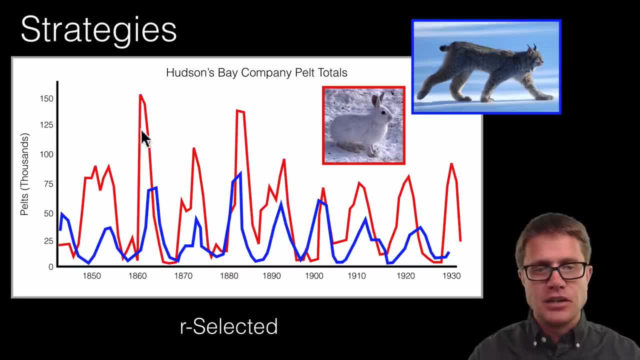 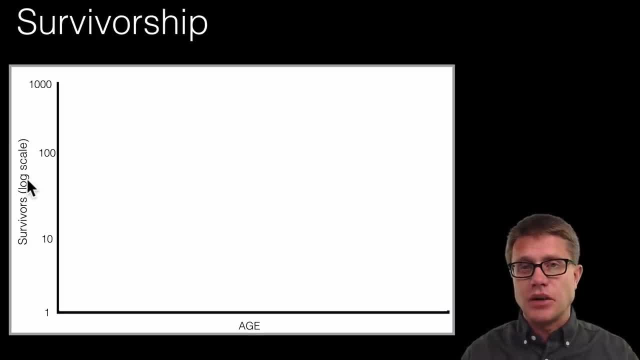 relationship where, as the Arctic hare population increases, then we can have more lynx feeding on it. But as they crash, then the lynx are going to crash as well. Now, a way to look at which strategy species are using is figuring out their survivorship, And so we have time. 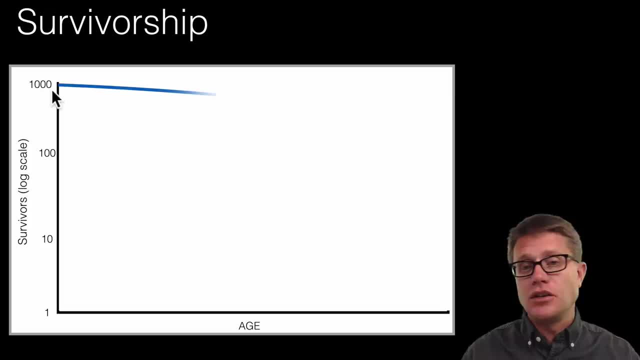 on the bottom And then we have the survivors on the side. So if we look at humans as a type 1 survivorship curve, what that means is when we are born, almost all of the humans survive, And then throughout their lifetime, almost all of the humans survive, And then 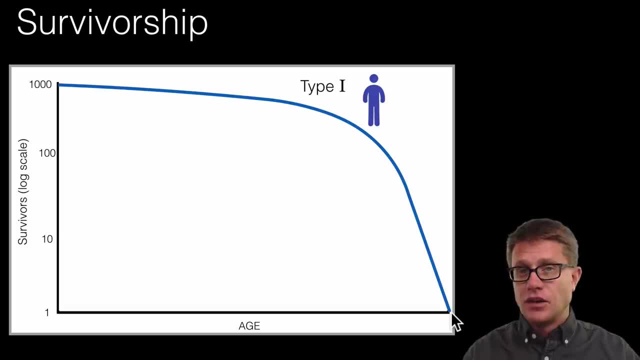 throughout their lifetime. almost all of the humans survive, And then throughout their lifetime they all die right at the end, And so we give a lot of parental care to our offspring. Almost all of them survive, And then when we get into our 80s, 90s, then we 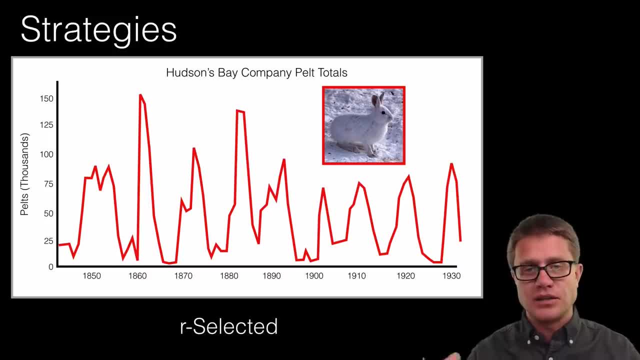 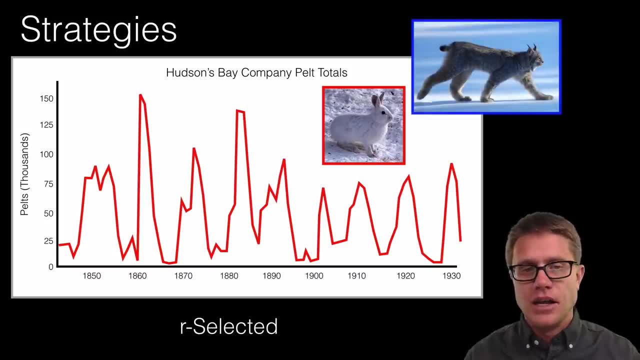 their population is going to increase and then it will crash. So we have this boom and bust cycle. Now what is interesting is that there is another species, And so the arctic hare are fed on by the Canada lynx. And if we look at their population, their population, 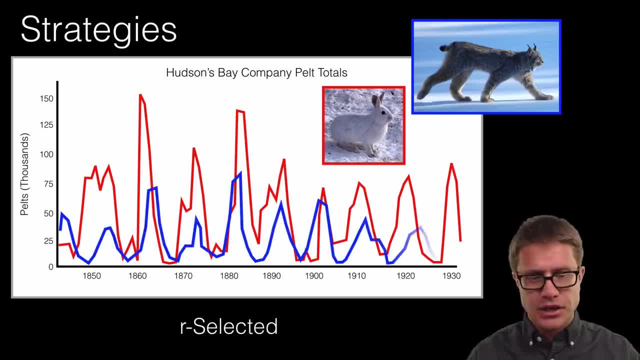 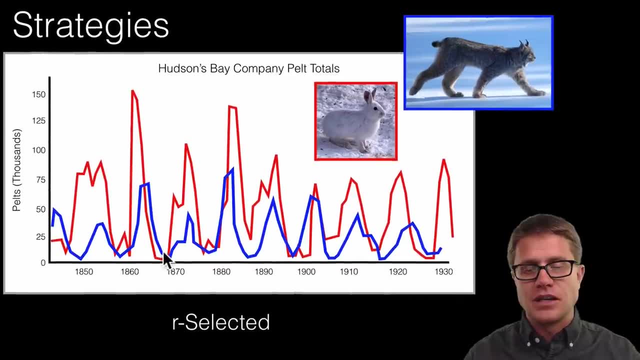 goes through a boom and bust as well. We have what is called a predator-prey relationship, where, as the arctic hare population increases, then we can have more lynx feeding, And that is feeding on it. But as they crash, then the lynx are going to crash as well. Now a way: 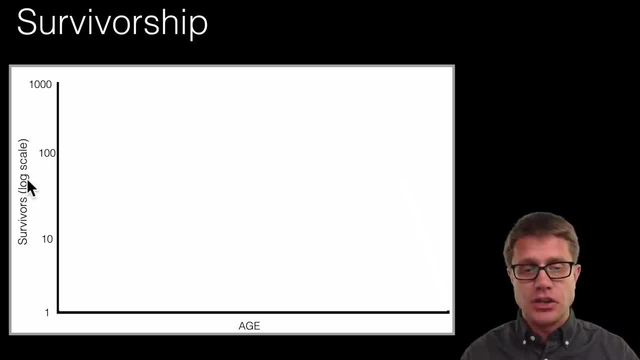 to look at which strategy species are using is figuring out their survivorship. So we have time on the bottom and then we have the survivors on the side. So if we look at humans as a type 1 survivorship curve, what that means is, when we are born, almost all of the humans survive And then throughout their lifetime they all die right at the end, And so we give a lot of parental care to our offspring. Almost all of them survive, And then when we get into our 80s and 90s, then we all die off. 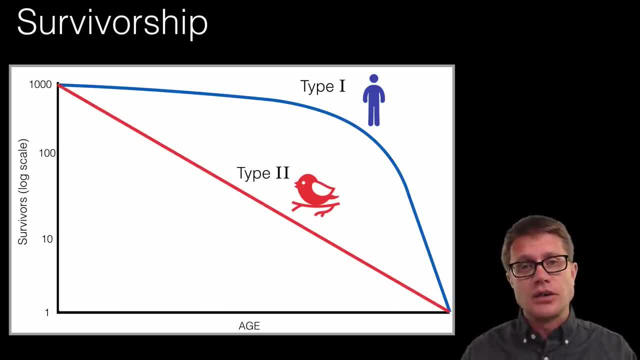 We could also have a type 2 survivorship curve. Songbirds are an example of that. From the moment they are born, they are dying off at a constant rate. Or we could look at type 3.. Those are individuals like the acorns from a tree. Almost all of them die, but a few. 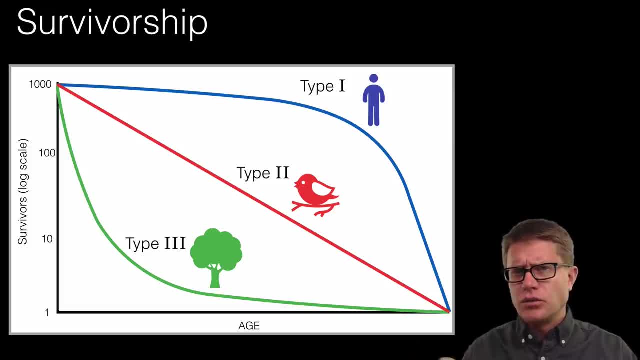 of those survive and those make up the plants that we have. And so could you link that to K or R selected species. Well, type 1 individuals are generally going to be those K selected species And then type 3 are generally going to be those R selected species. But there 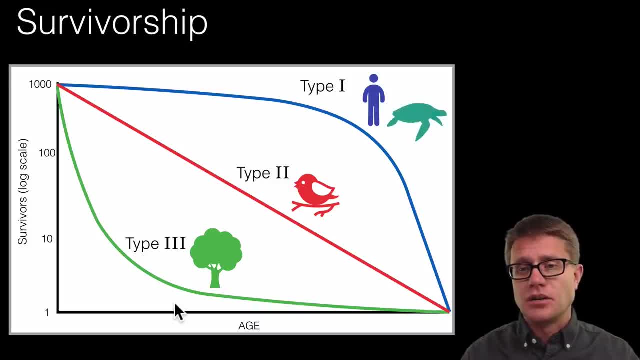 are so many examples that are in the middle. So if you think about a sea turtle, for example, they have lots of offspring, They do not give much parental care, but they live a long time, And so it is not as simple as R-U-R or R-U-K. It is somewhere in the middle, But they are. 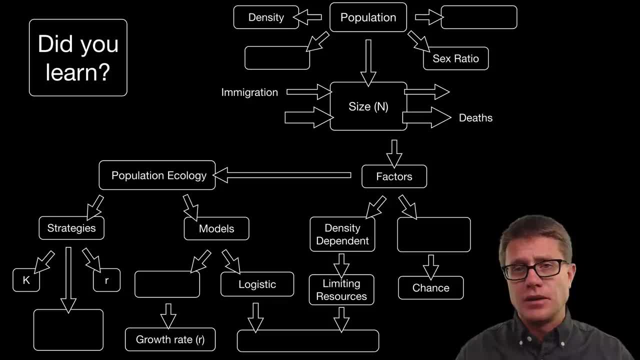 applying these different strategies in life, And so did you learn the following. Could you pause the video at this point and fill in the blanks? If not, population size is determined by immigration and birth. That increases it Decrease by immigration and deaths. We have got other characteristics: Density distribution. Density distribution. 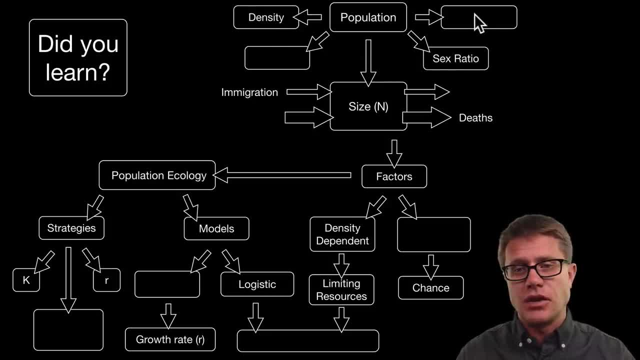 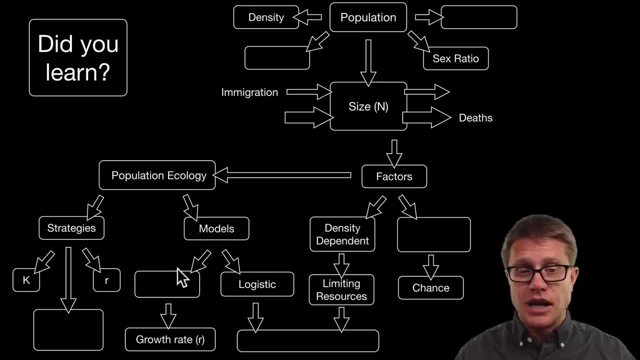 carrying capacity or K, We use models to study it. Exponential models are built on the growth rate, Logistic models also built on the growth rate, but include carrying capacity. And then we have different strategies in species: K selected, R selected. Remember, we are K selected. 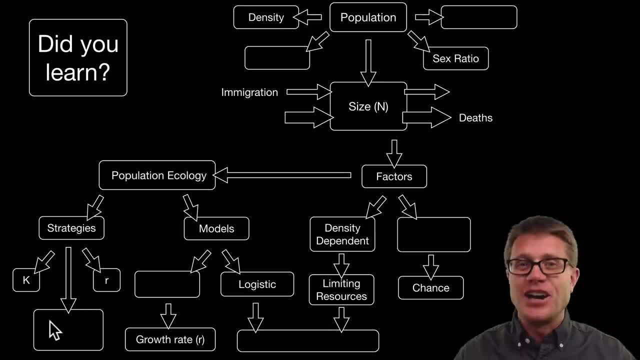 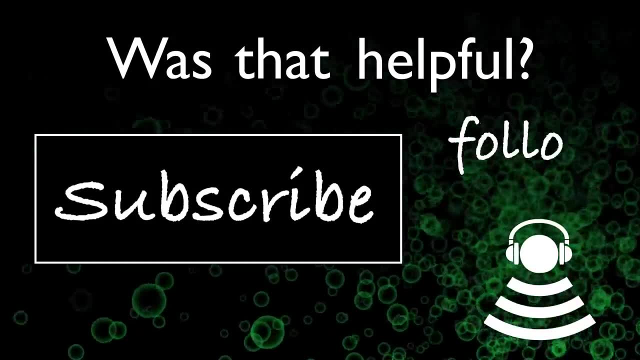 And then we have survivorship curves that we can study to get that. That is a lot. I hope it made sense and I hope that was helpful. 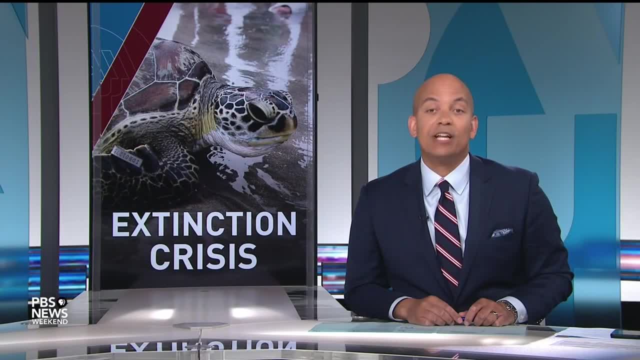 Globally, one in five reptile species is facing the threat of extinction. That's according to a recent study in the scientific journal Nature. We take a deeper look now at what's driving this extinction crisis and what it could mean for the rest of the world. 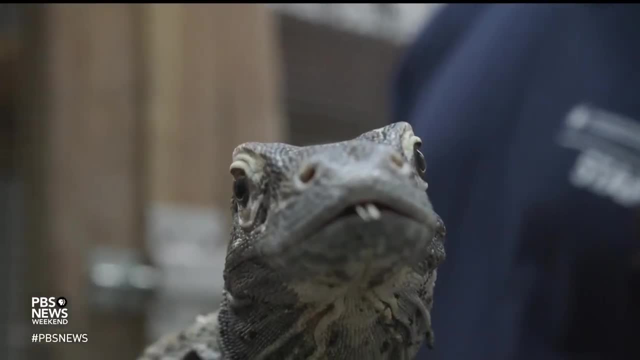 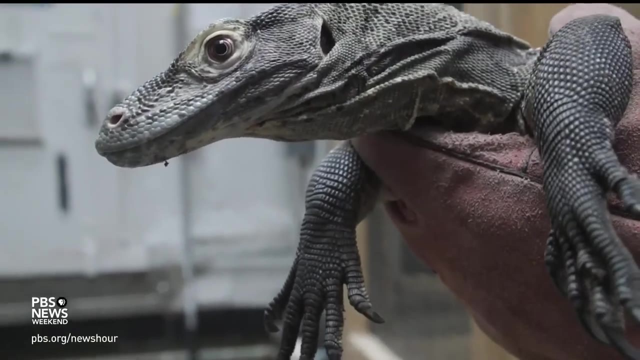 So this is Onyx. This is a two-year-old male Komodo dragon. On a recent day at Smithsonian's National Zoo in Washington, we met Onyx, a juvenile Komodo dragon. They are the world's largest lizard, often growing up to 10 feet long. 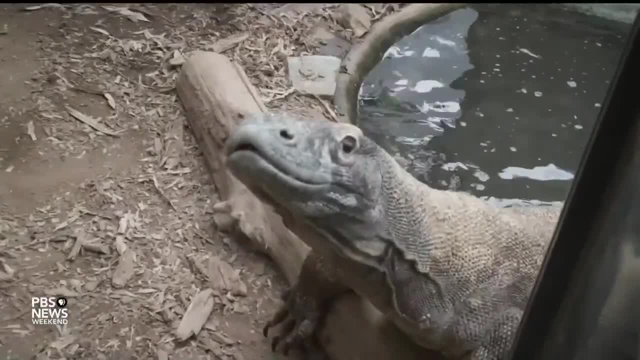 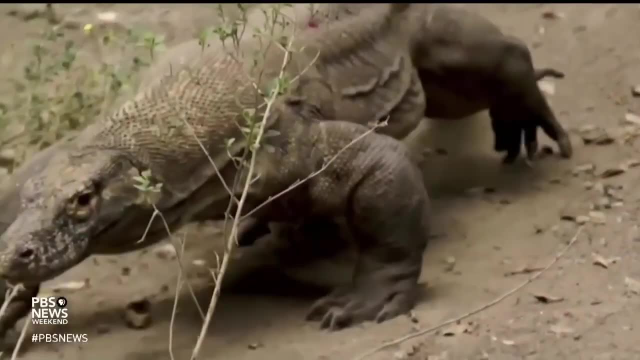 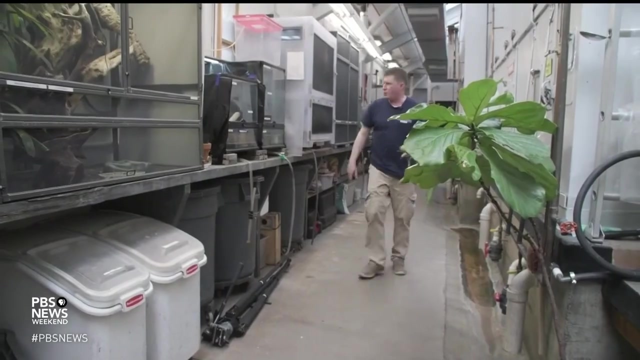 with some weighing more than 300 pounds. Native to a few islands in Indonesia, these incredible reptiles date back one million years, But because of habitat loss, Komodo dragons are now facing an uncertain future, says Matthew Evans, an assistant curator at the Smithsonian's Reptile Discovery Center. 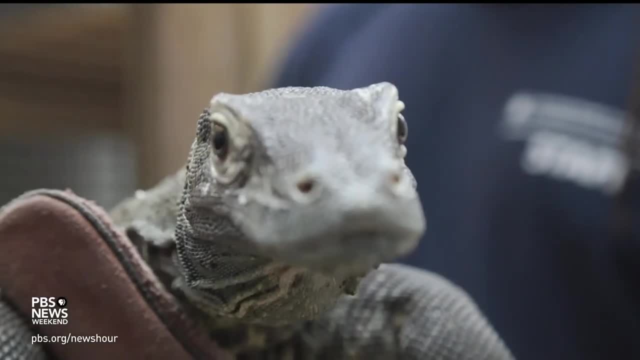 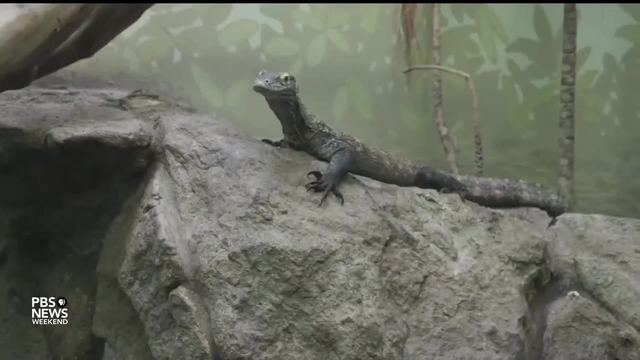 MATTHEW EVANS, Smithsonian's National Zoo and Komodo Dragon Research Center. Smithsonian Komodo dragons are endangered And these guys are part of a species survival plan. That plan is part of a larger effort here at the National Zoo to highlight why reptiles are vital to our entire ecosystem- Komodo dragons. we call it kind of a keystone species. So if you remove them as a top predator in the environment, the rest of that ecosystem doesn't function right. They actually need that top predator for all the roles that it plays with creating habitat for keeping. 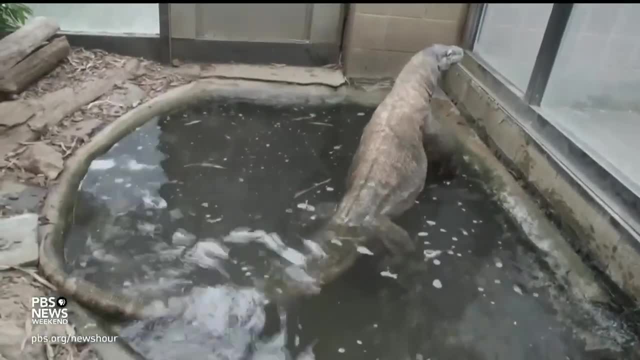 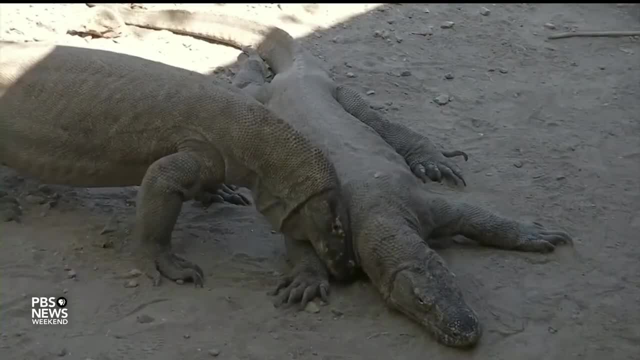 if they disappear, there's a domino effect. The plight of the Komodo dragon is not unique, says zoologist Bruce Young, who recently co-authored the largest global reptile study of its kind. BRUCE YOUNG, ZOOOLOGIST KOMODO DRAGON. Our goal was to assess every single species.